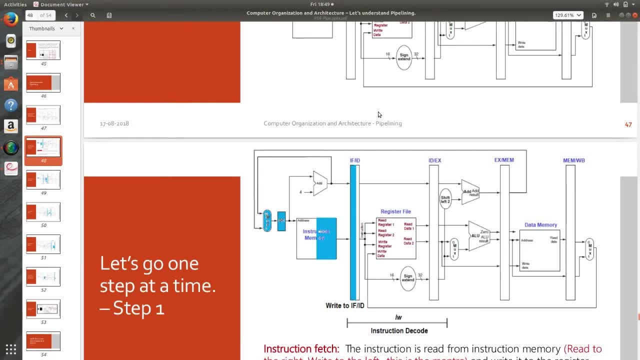 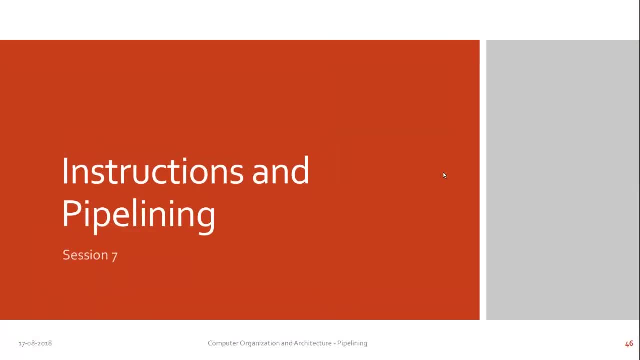 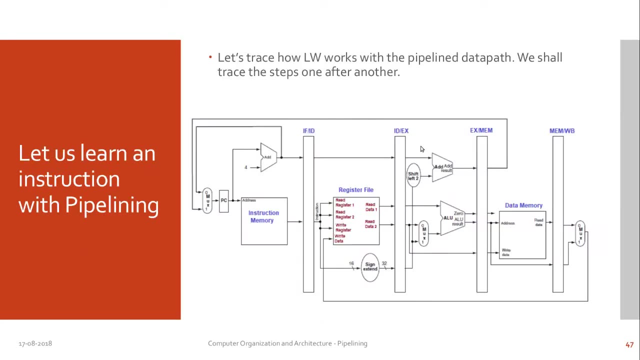 Friends, in my previous session I spoke to you about the need of registers in the pipelining stages and, most importantly, how exactly the registers are used. All these things I clarified very clearly in the previous session. In this session I am going to talk about how to trace the data path in the pipelined data path model. For example, if I have to trace the way an instruction is working, I need to do it appropriately. Now you can see that here I have got IFID register in between. Meanwhile I have got IDEX register in between. I have got EXMEM, I have got MEMWB. So how it works, how do we trace it? 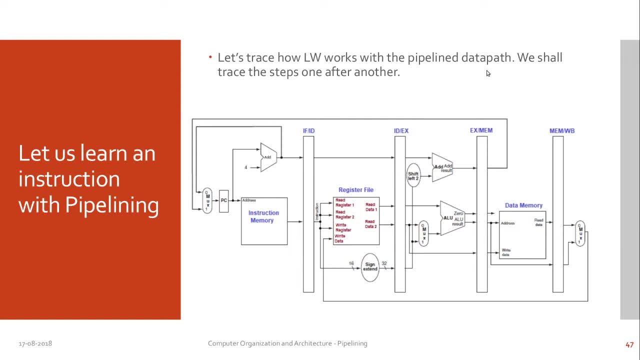 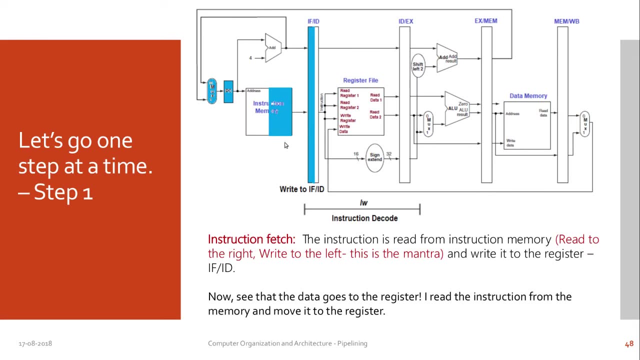 I am going to trace the instruction load word from this. This is a datapath with pipeline, So please understand. whenever I have to represent the right, I need to highlight the left part of the register. Please understand. the right goes left, The right goes left. I repeat: Whenever you have to read, you need to read from the right. The read goes in the right. Now, what are the stages in the instruction? 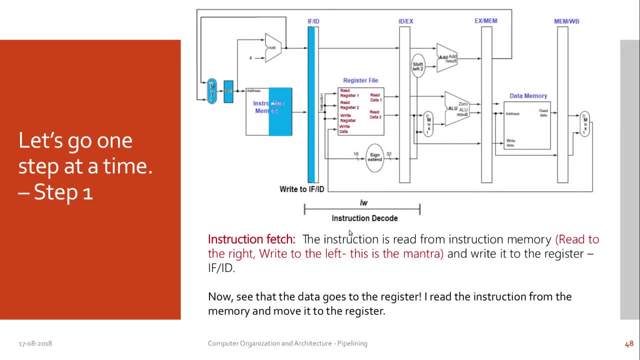 The first stage is instruction decode. So what do you do? It is very simple. stage is to fetch the instruction. i mean the instruction fetches the first stage. and you can see that here i am fetching the instruction. fetching is nothing but reading the instruction. 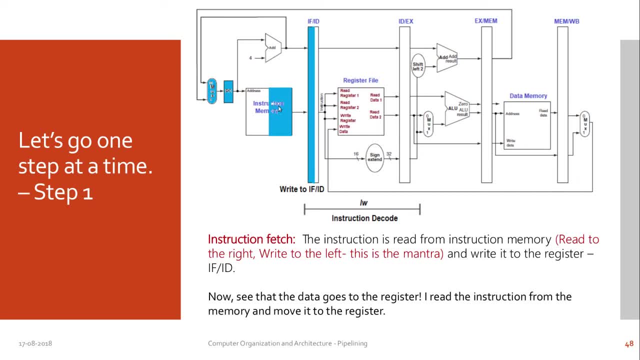 so the multiplexer is completely used, the pc is completely used and i read the instruction. hence i read it from the right and then i write it into the intermediary register if and id. so whenever i write, it goes to the left. please remember. when i write, it goes to the left. so i have read the 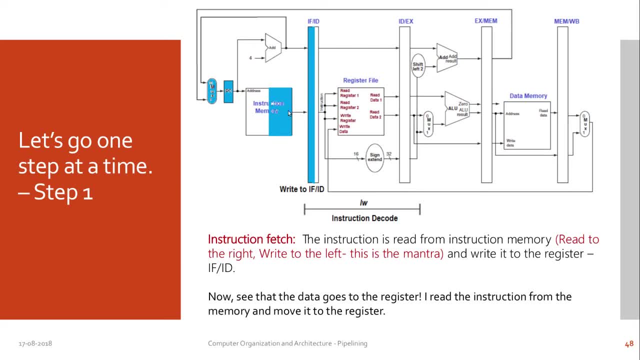 instruction from instruction memory. it is represented by a right side. i have written the instruction into the if slash id register so i represented by highlighting the left side of the register. this is the first step in the tracing. this is very important. let's go to the second. 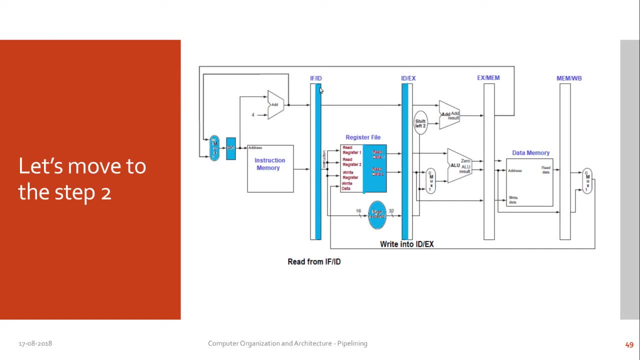 step. now. i need to read the content from if id. so i am going to read the content from if id. so i need to highlight the right hand side. this is wrong. this should not be highlighted, so please don't take it otherwise. this is wrong. this, this has to be corrected in the ppt, so don't worry about it. this is wrong now. 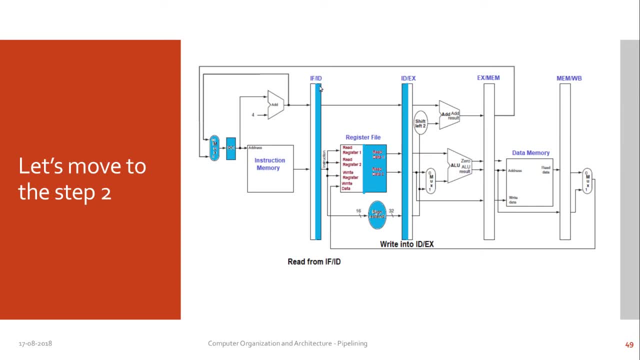 the if and id has to be the register content. if and id has to be read now. so when you have to read, it goes in the right. so i read the content from it and i understand that i need to use this particular registers and i read the content from the registers also, since it is a load. 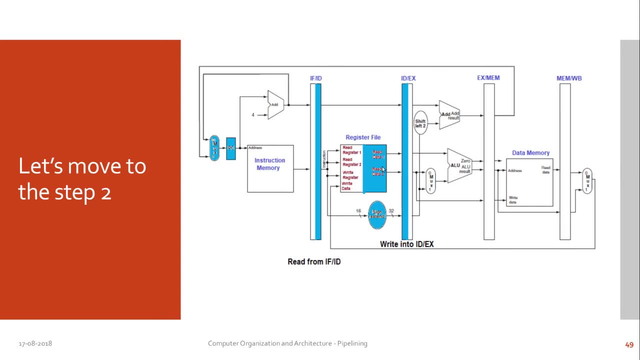 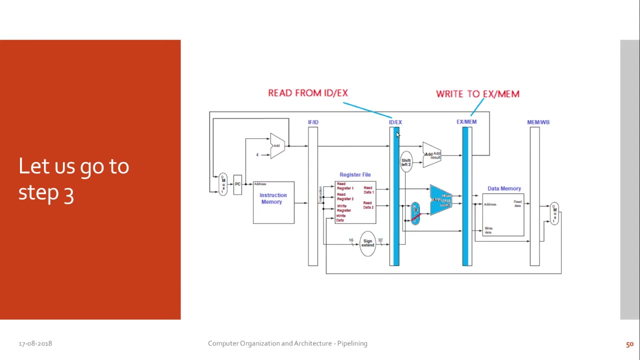 word instruction. i will use the sign extend completely and then i will write the content into the id ex register. so i write: it goes to the left. so you can see that here. i have written the content into the left now. so what is the third step? it's very simple. i have now got the content into idex, so i need to read. 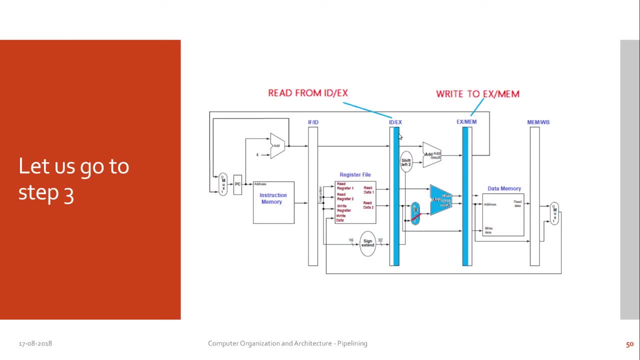 from it and then i need to move it into the alu. so i have read from it, so reading happens in the right, so i read from it and then i push it on to my multiplexer through one and i use the alu completely and the results are to be returned into the memory. ex memory register is the one. 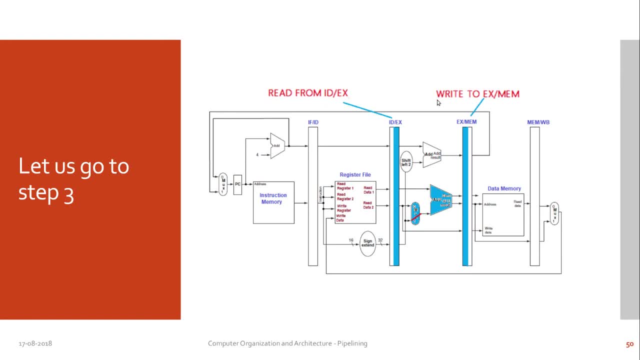 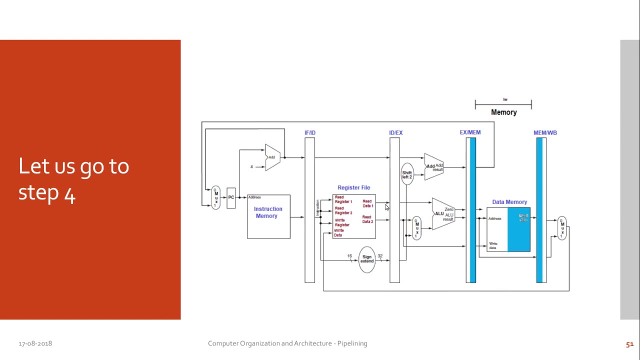 that we are going to write into now. very simple: i have taken the content from idex. i have written the content into ex mem. that's it. when you write, you need to do it in the left. when you read, you need to do it in the right. please don't forget now i what is load word? load word is all about. 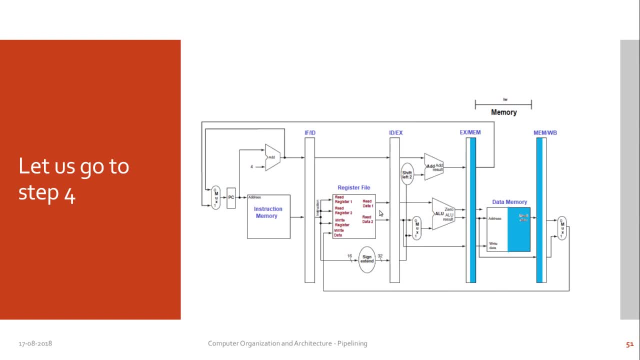 loading a particular content into a register. but the address where from the content has to be retrieved is to be calculated through the alu operation and that content is to be read from the data mem location. now, here i would have got the address and the address is used to read the content from. 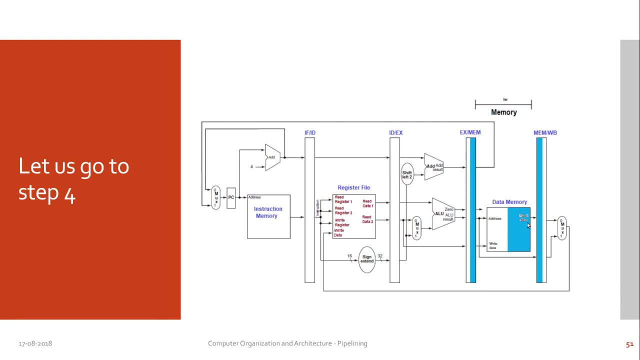 the location. so i'm going to read from the right and i'm going to write into the left. the mem read back the write back stages here. i'm going to retrieve the content from the memory location and i'm going to write it into this register. so this register, mem and wb has got the content now. 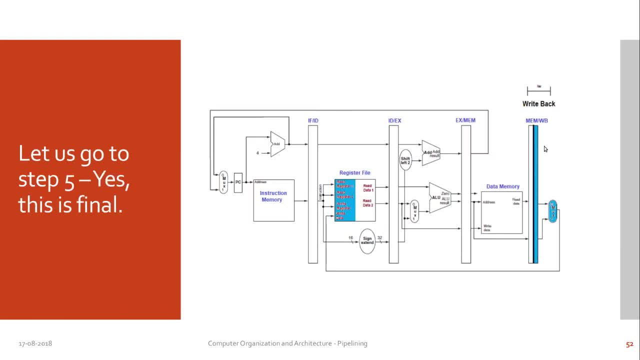 now the next stage is very important. what i'm going to do here is i'm going to write it back, so i need to read it from the mem wb register and i use this multiplexer. i will send the content via this way and i am going to. 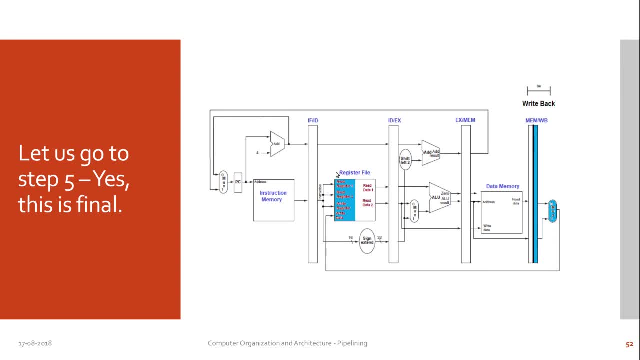 write it into the register file. the right happens to the left, read happens to the right. now what have we done is very simple. we have used the registers, we have read from the right, we have written to the left, we have taken the content from the instruction memory, we wrote into the.